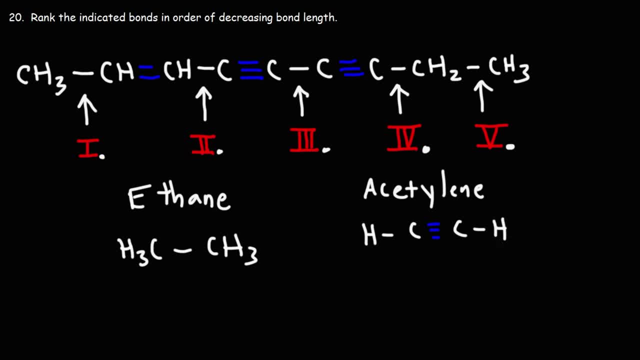 They're shorter than single bonds. But now let's include hybridization into the discussion. If we look at what type of orbitals are overlapping to form the single bond or the sigma bond, these are sp3 hybrid orbitals. Each carbon in ethane is sp3 hybridized. There's no 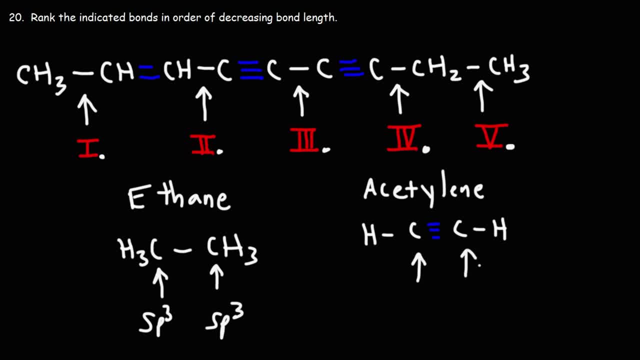 pi bonds. Now in acetylene we have a triple bond which means there's no pi bonds. So we have a triple bond which means there's no pi bonds, And those two carbons are part of you know. they both have two pi bonds. 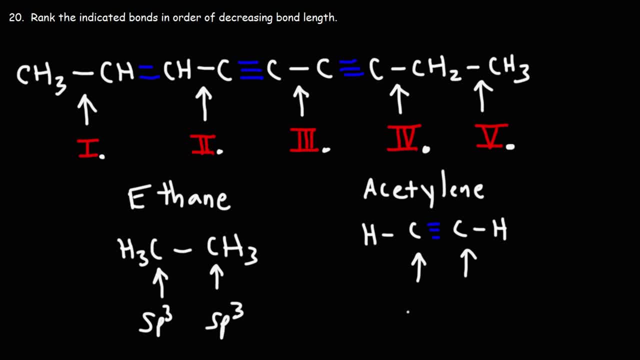 So for one pi bond it's sp2 hybridized, But for two pi bonds it's sp hybridized. So the triple bond is formed from the overlap of two sp hybrid orbitals. Now how much s character is in an sp3 hybrid orbital? So to make an sp3 hybrid orbital, 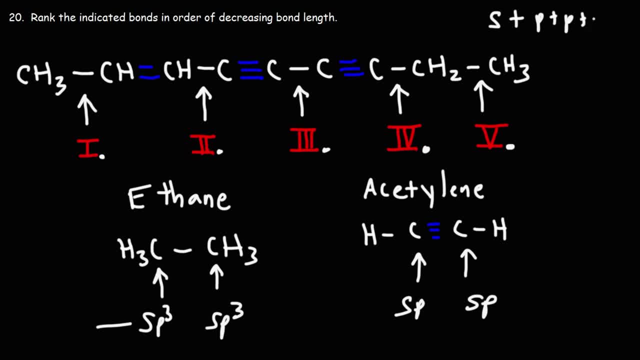 we've combined one s orbital with three p orbitals, So we have one s out of a total of four orbitals. one out of four is 0.25 or 25%. An sp3 hybrid orbital has 25% s character and it's 75% p. 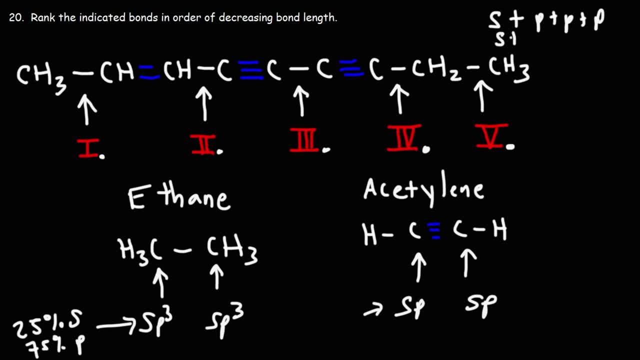 An sp hybrid orbital. It's a hybrid of 1s and 1p, So one out of two orbitals is 45% s character and 75% pi. So an sp hybrid orbital has 25% s character and only 75% pi. 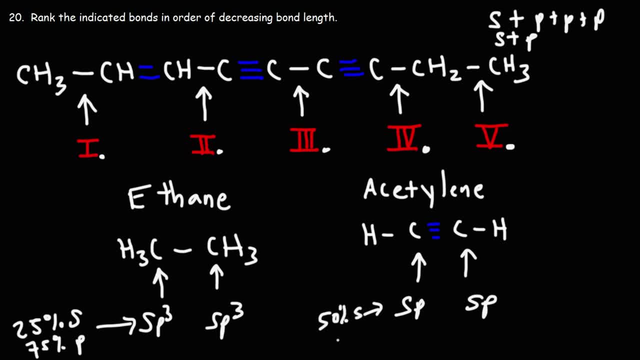 An sp hybrid orbital has 1p. 1 p digitized and preceded by 2. Hibd can be saw at these factors, One out of two orbitals. it's 50% S and 50% P. So the reason or one of the reasons why acetylene is a shorter bond, let me say this again. 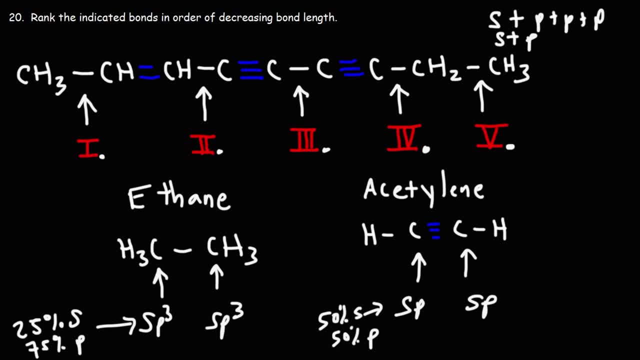 The reason why a triple bond is shorter than a single bond is because it has more S character. Now we have to be comparing atoms in the same row, Because if you're comparing an atom in a different row, like iodine versus fluorine- 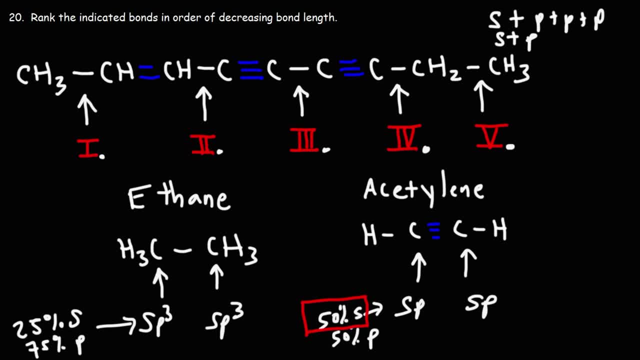 now you're looking at different energy levels. Fluorine is in the second energy level, iodine is in the fifth energy level, And so that's a whole different story. But here we're looking at carbon atoms in the same row of the periodic table. 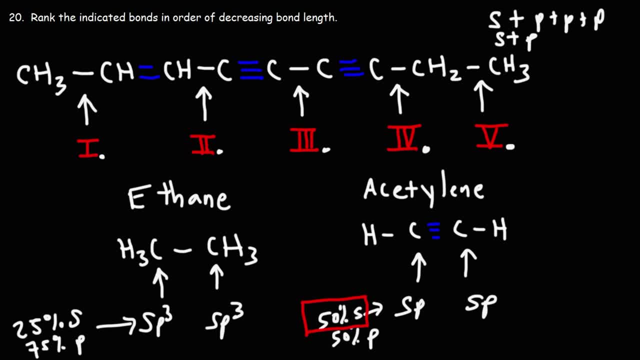 So when comparing elements in the same row that are close to each other, we need to look at S character. The more S character there is, the shorter the bond is going to be and the stronger the bond will be as well. Now, the reason is that the S orbital is closer to the nucleus than the P orbital. 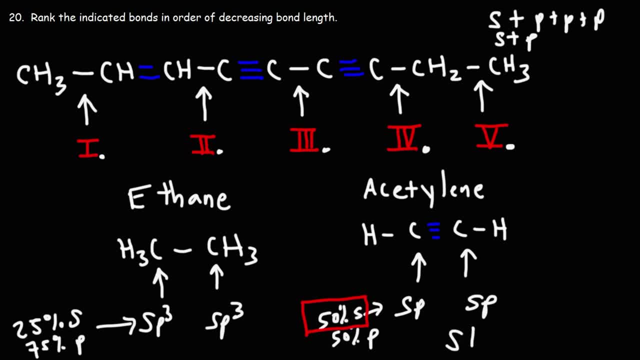 So that's why, as the S character increases, the bond strength will increase, but the bond length will decrease, And that's how we're going to figure out which one of the single bonds is the longest and which one is the shortest. The shortest ones have more S character. 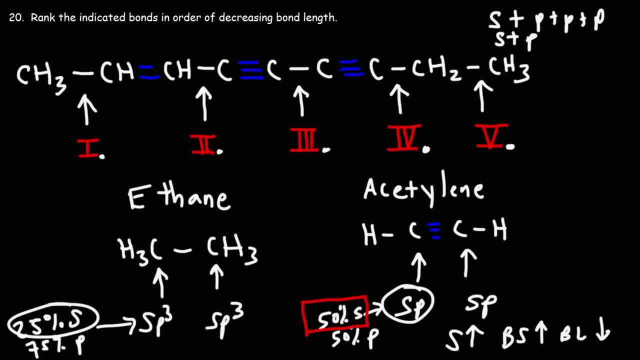 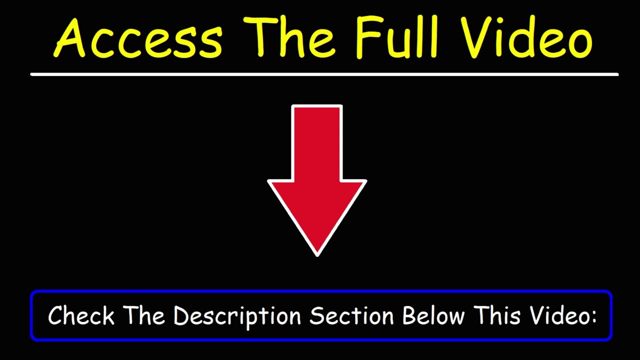 The longer ones have less S character or more P character. So we need to determine the orbital overlap of each bond, In other words the hybridization of the atoms that make that bond. Now for those of you who are interested in getting the full video with all 90 practice problems: 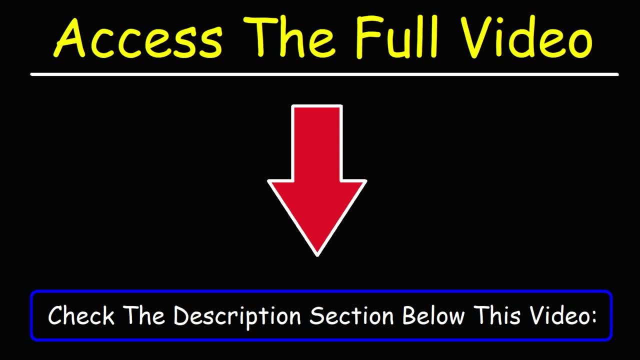 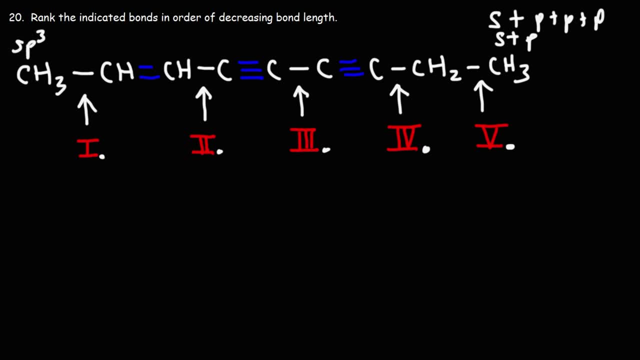 feel free to check the description section below this video. So this is an sp3 hybridized carbon, This is an sp2 carbon, This is sp2.. The triple bonds: they're associated with sp hybridized carbons And the last ones, the CH2 and the CH3 carbons, those are sp3 hybridized. 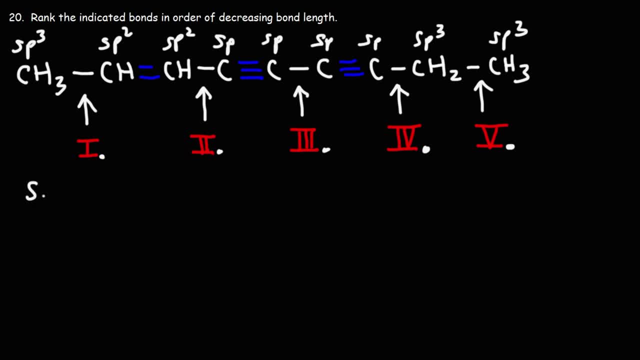 So bond number one: it's formed from the overlap of an sp3 hybrid orbital and an sp2 hybrid orbital. Now this single bond number two is formed from the overlap of an sp2 hybrid orbital and an sp2 hybrid orbital And an sp hybrid orbital. 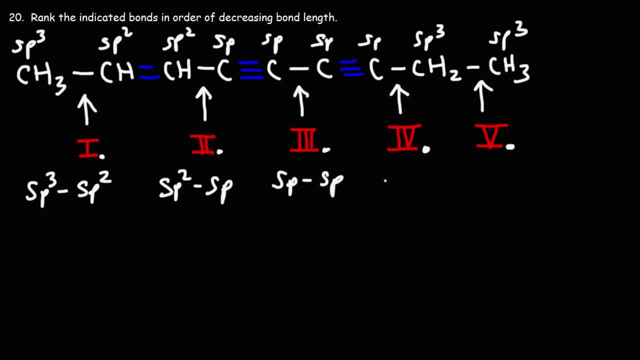 For number three, it's sp, sp. Number four, sp, sp3.. And number five, sp3, sp3.. So remember, the more S character that we have, the shorter the bond. So S is going to be shorter than sp, which will be shorter than sp.